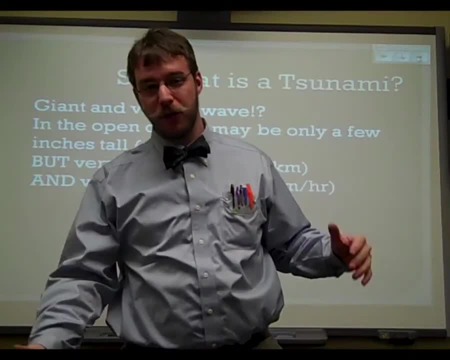 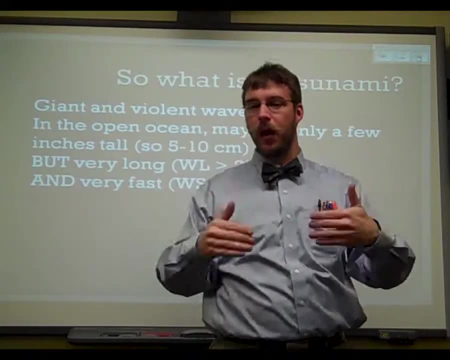 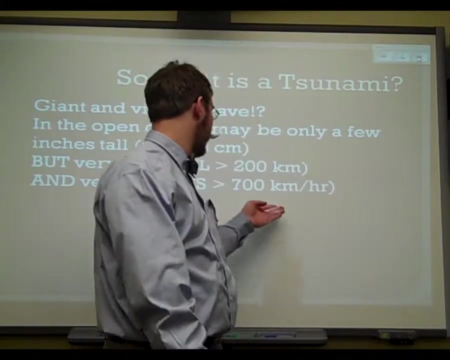 little, But they have a super long wavelength. On average, the wavelength for these waves will be over 200 kilometers. In addition to that, the wave speed is very fast. The movement of the wave, it actually moves. Each crest of the wave will move in about 700 kilometers per hour, which is, yeah, that's fast, like airplay. 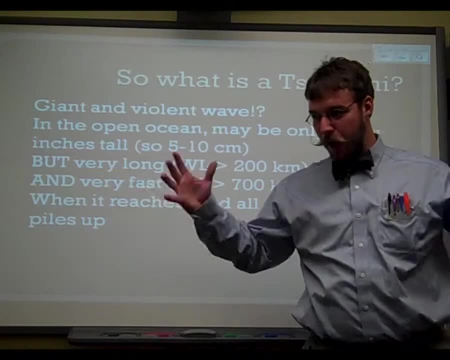 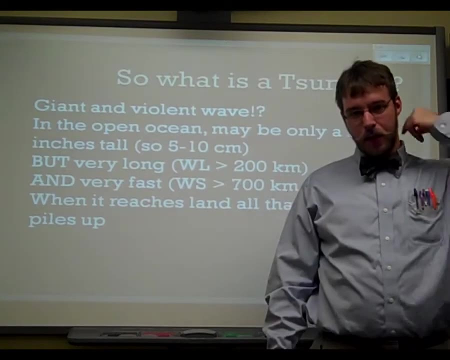 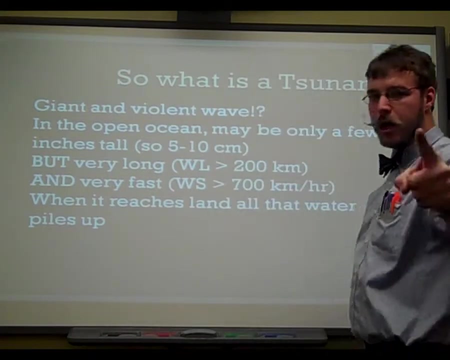 Fast. When it reaches land, you've got all that water spread over. that big, long wavelength tends to pile up on itself and that's when they get big and terrifying Again, because it's coming into a shallow area that is affected by tides and tidal waves. A lot of people call it a tidal wave, but still not a. 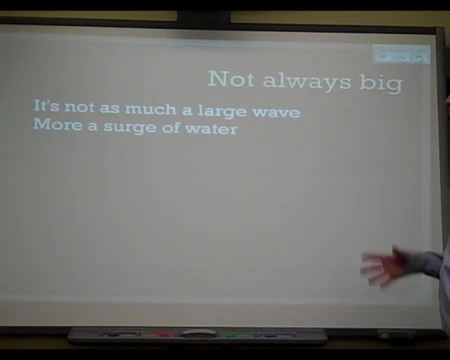 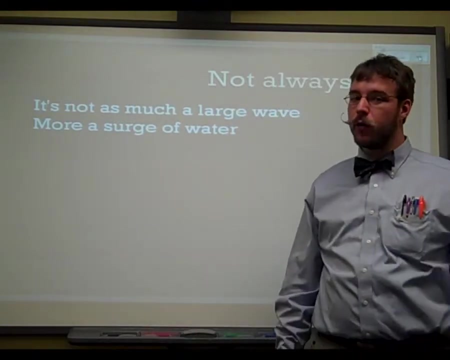 tidal wave. So I don't want you guys to think of tsunamis as a large wave as much as a huge surge of water. Think of it like the storm surge that comes from a hurricane and it reacts and piles up, coming in the land in a very similar way. 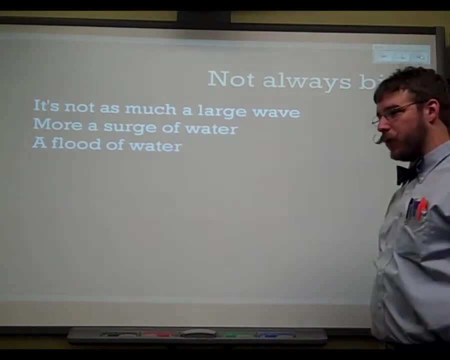 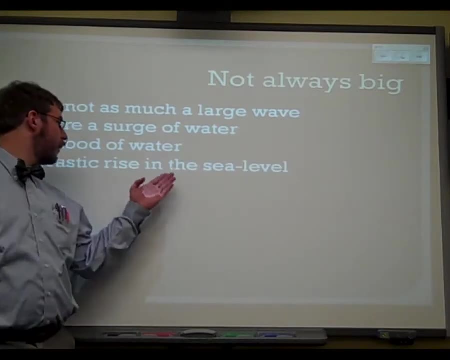 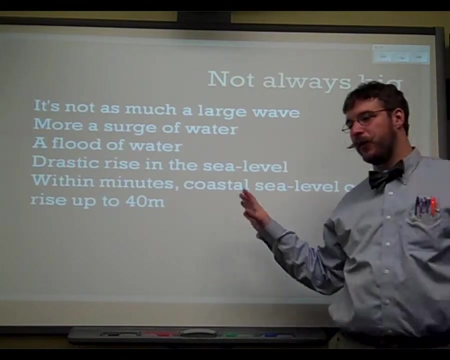 It's a flood. of water Floods the area, Destroys everything. That's the badness. As a result, you get these drastic increases in sea level Within a matter of minutes. the coastal sea level in the event of tsunami can raise 40 meters. The 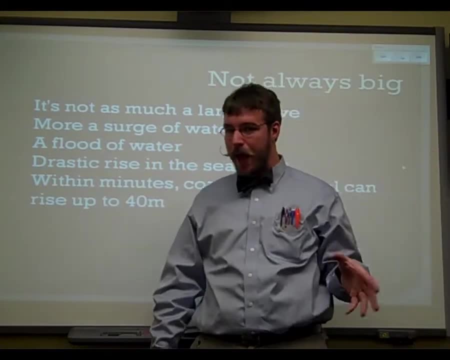 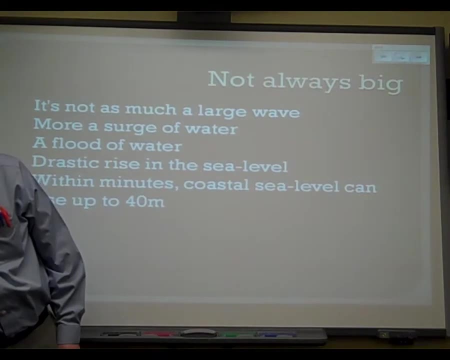 super high-end dive that we're going to talk about in a minute is going to be a lot of people can break their neck off. of is 10 meters, All right. so this is four of those piled up on the top of each other, If you give you a little. 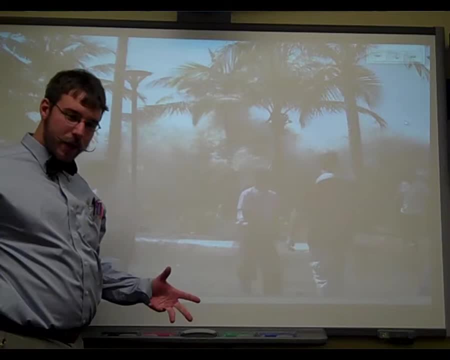 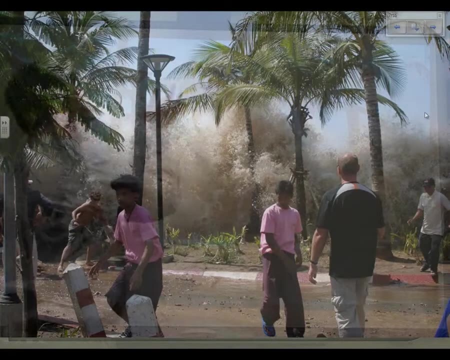 perspective And after all that, this is what you see. These are people, These are palm trees. That is a giant tsunami coming on the shore and well, yeah, these people are probably not going to have a good time. Here's some more pictures This is showing you. 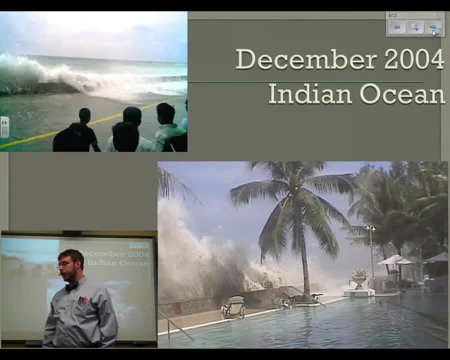 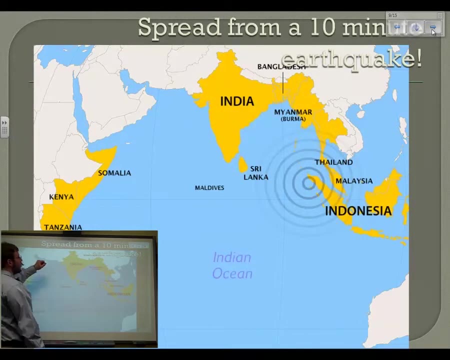 the Indian Ocean storm surge coming in in 2004.. There was a huge tsunami right when I graduated from high school. Here is the seawall: It's coming up into this resort. That was bad. Here is that same thing and actually spread from. 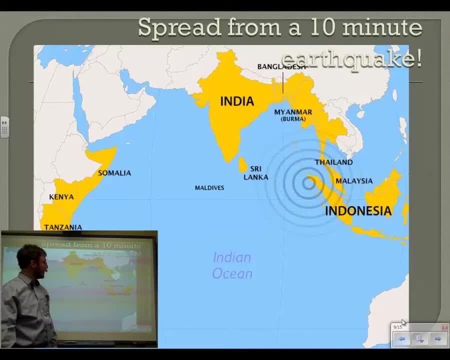 earthquake that lasted about 10 minutes. Right here next to Indonesia. You got some plate tectonic action And remember we talked about how waves can be formed from drastic changes underneath the seafloor- Tsunamis are the ones that come from that sort of thing. So you can see, you got this earthquake, that focus. 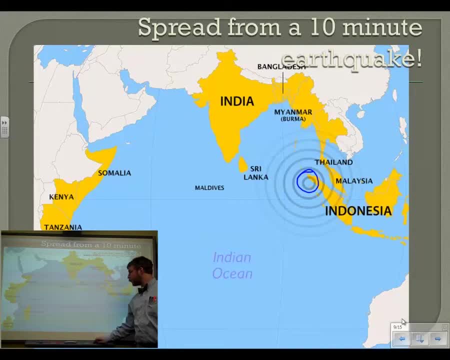 on this area right here And, as a result, the water spread and that elliptical, on that circular wave pattern. Not an orbital wave, This is different. This is a big old tsunami wave just spreading out through the entire ocean And pretty much all of this got smashified in the smasher zone. 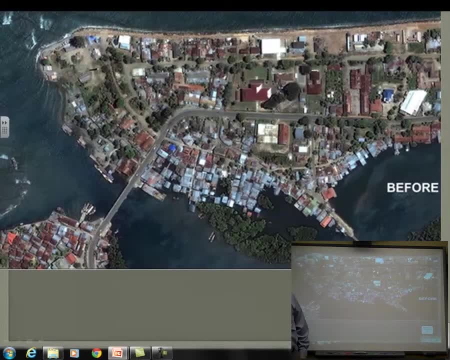 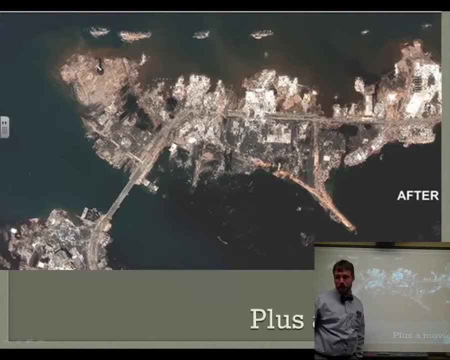 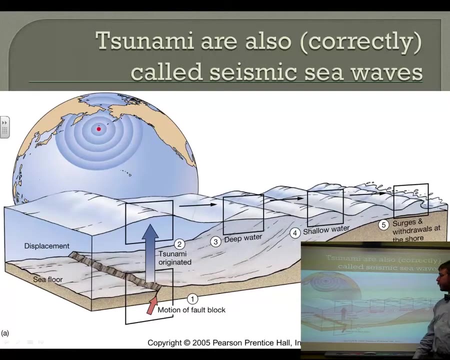 Here's a before and after picture, Before the tsunami comes in picture. And here is the after. Notice how the yeah, that's bad, That's bad. So the technical term for tsunamis are the seismic sea wave. Here's a nice diagram that shows pretty much what I just talked about. You have a motion. 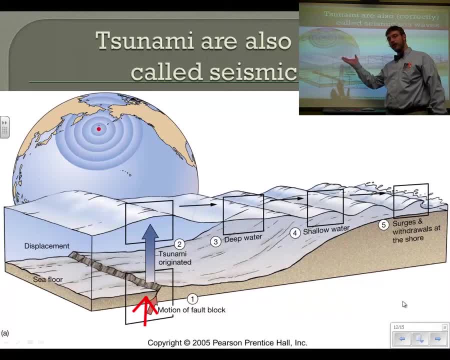 from faulting either dropping or rising. that causes a huge displacement in the water. It bubbles up and it spreads in 360 degrees. This is just showing you one of the waves, And in deep water it's pretty small. This is really over exaggerated. In shallower water it starts to pile up And then when 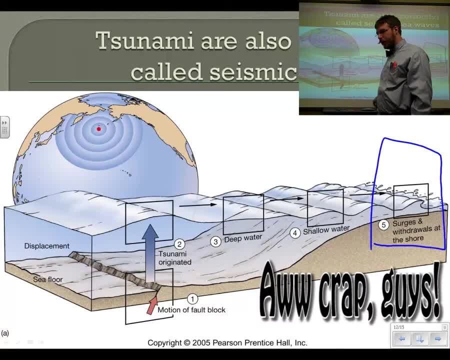 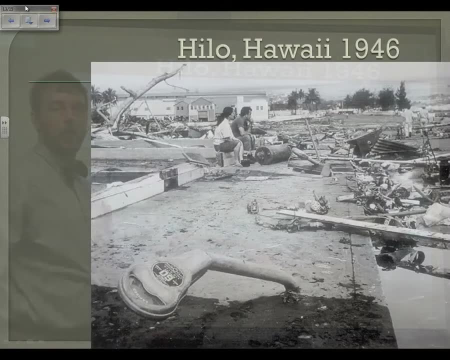 you hit the shore, that's where the badness comes in. It piles up on that continental shelf and makes huge waves. you know, 40 meters and up, Here's a tsunami that hit Hilo, Hawaii in 1946. And you can see that this is a parking. 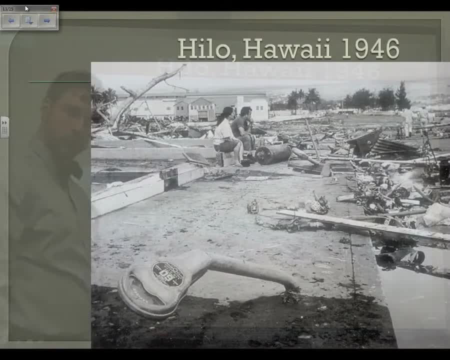 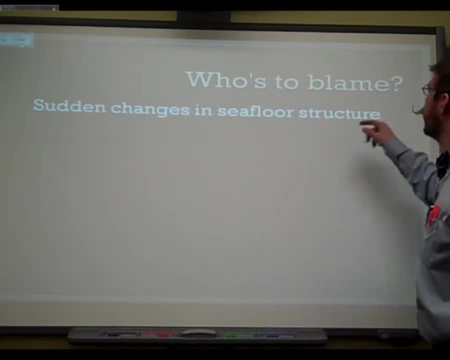 meter that got bent. That's a tsunami that hit Hilo, Hawaii, in 1946. And you can see that this is a parking meter that got bent. Ah, so much power in the water. So who's to blame for the tsunamis? There's a sudden change in the sea floor. That's what. 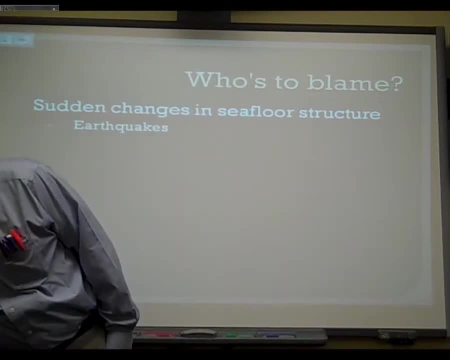 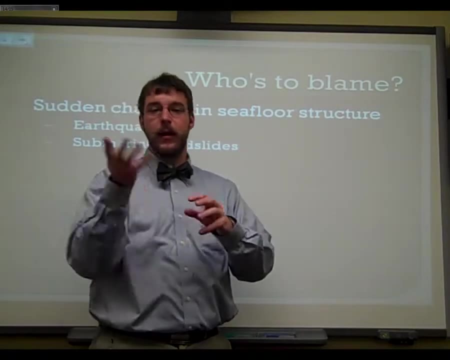 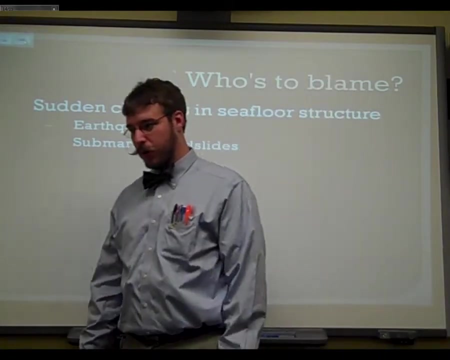 will give you a little tsunami action. Earthquakes are therefore to blame, And also submarine landslides. Any time you've got on your continental slope, a big turbidity current comes through. that can actually kick off a little bit of a sudden change in the sea floor as well. Even down in the deep sea tropics, there's a lot of sudden change in the sea floor as well. Even down in the deep sea tropics, there's a lot of sudden change in the sea floor as well. Even down in the deep sea tropics, there's a lot of sudden change in the sea floor as well. In the eastern trenches. volcanic eruptions are another one, Basically any event that causes the volume of seawater to a shift, Not usually at strike-slip faults, since those are more of a horizontal movement. We're looking for areas of vertical movement, which means you guessed it all that plate.